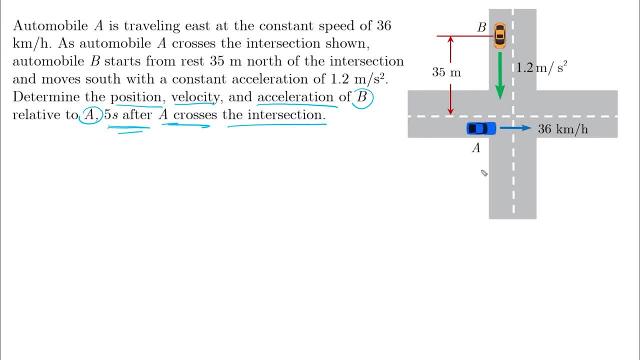 So clearly we will be using here constant acceleration equations, because all values here are constant and the problem is asking for position: acceleration rb relative to A, velocity vb relative to A and acceleration ab relative to A after five seconds. 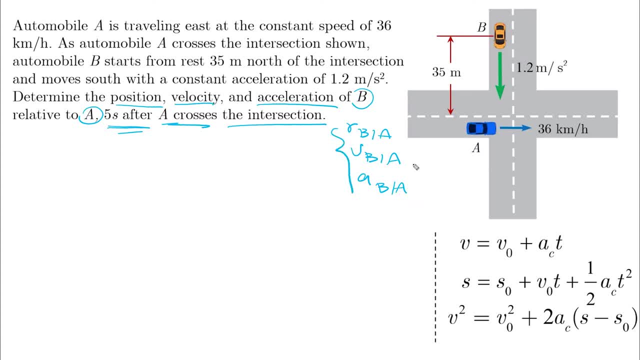 So we need all variables for A, all variables for B, and then we just subtract them from each other And let's start with this diagram so we can understand what is happening. So this is the position vector of A, the position vector for B, and this is where B is starting from 35 meters. 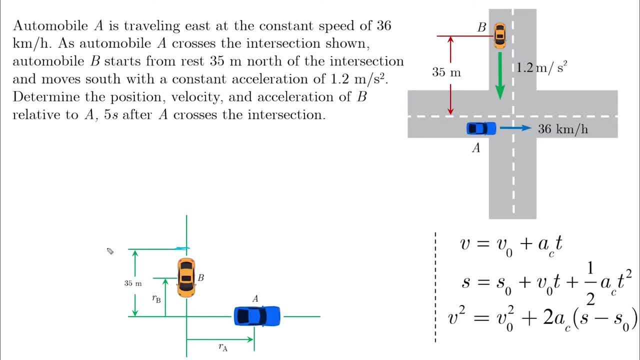 So rb initial will be 35 meters and it is starting from rest with 1.2 meters per second square. Now for the horizontal car. it has a zero acceleration, So AA is equal to zero And it has a constant speed which is 36 kilometers per hour. 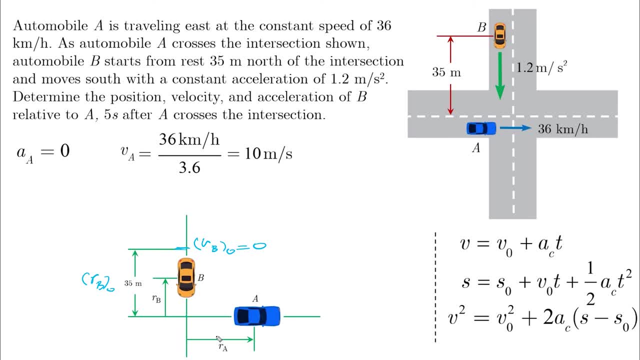 And if we divide this by 3.6, we get 10 meters per second. So for car A we will be using the second equation, with A equals to zero. So this becomes S equals S naught plus V naught T. 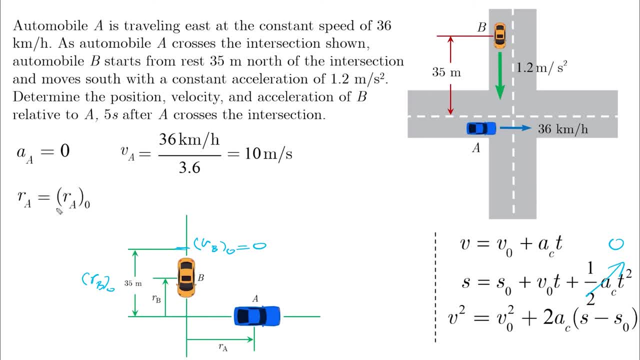 Or in our terms, RA equals RA naught plus VA, And this leads to 50 meters after five seconds. So after five seconds, A will be 50 meters to the positive right direction. And as for car B, we have its acceleration, which is minus 1.2 meters per second square. 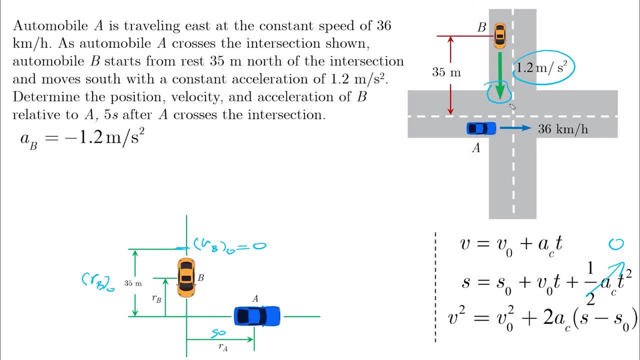 And we're taking this as a minus because we are assuming that RA or the position vector is positive up, So AB is down, which is minus, And since we have the acceleration and we have the initial velocity, which is from rest. 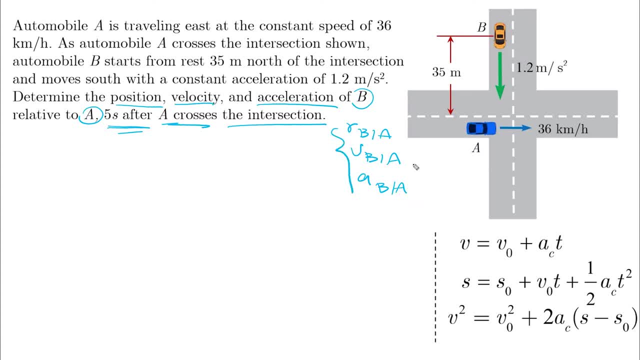 So we need all variables for A, all variables for B, and then we just subtract them from each other And let's start with this diagram so we can understand what is happening. So this is the position vector of A, the position vector for B, and this is where B is starting from 35 meters. 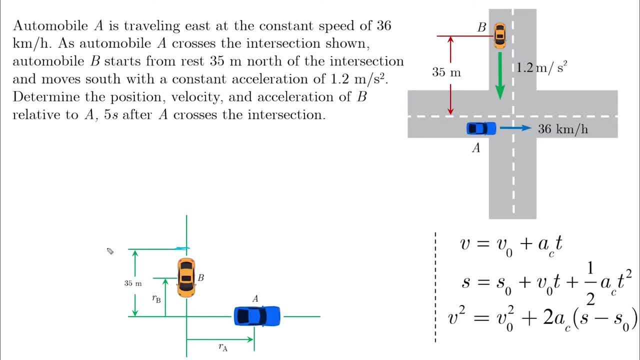 So rb initial will be 35 meters and it is starting from rest with 1.2 meters per second square. Now for the horizontal car. it has a zero acceleration, So AA is equal to zero And it has a constant speed which is 36 kilometers per hour. 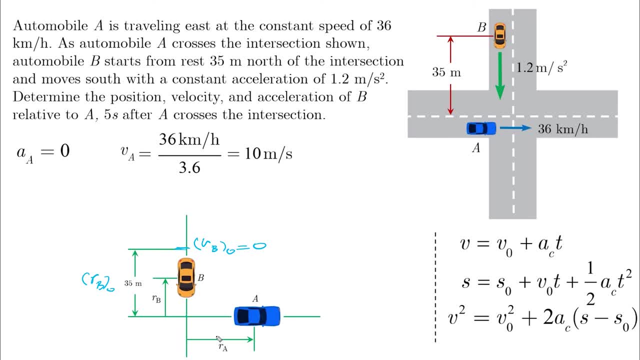 And if we divide this by 3.6, we get 10 meters per second. So for car A we will be using the second equation, with A equals to zero. So this becomes S equals S naught plus V naught T. 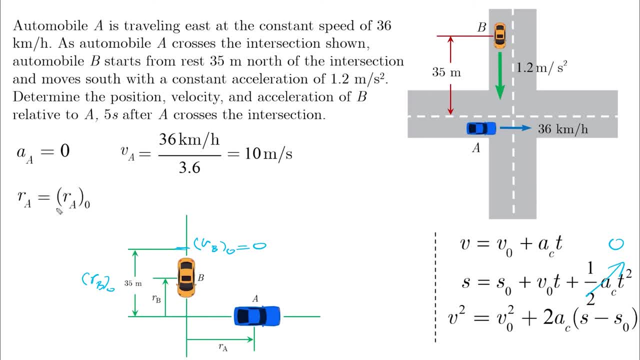 Or in our terms, RA equals RA naught plus VA, And this leads to 50 meters after five seconds. So after five seconds, A will be 50 meters to the positive right direction. And as for car B, we have its acceleration, which is minus 1.2 meters per second square. 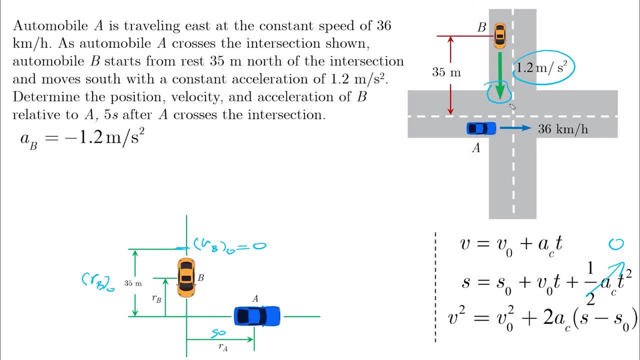 And we're taking this as a minus because we are assuming that RA or the position vector is positive up, So AB is down, which is minus, And since we have the acceleration and we have the initial velocity, which is from rest. 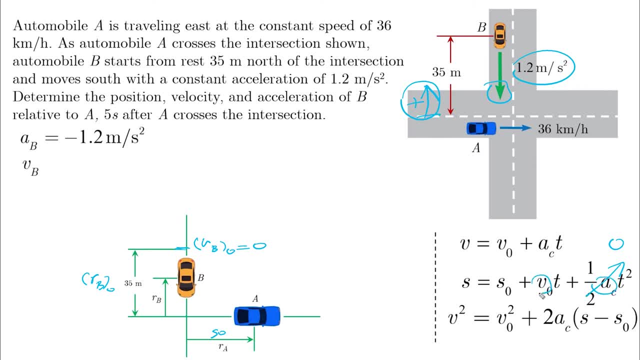 we can use the first equation and the second equation to find the velocity and the position after five seconds. So using the velocity equation, the first one, VB is equal to VB naught Plus AB times T, And this is assuming positive up. 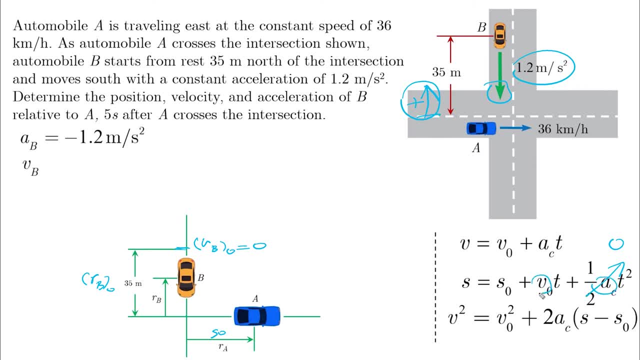 we can use the first equation and the second equation to find the velocity and the position after five seconds. So using the velocity equation, the first one, VB is equal to VB naught Plus AB times T, And this is assuming positive up. 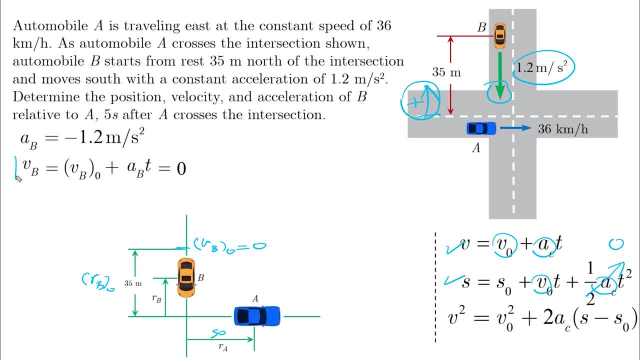 So we get zero from rest, Minus 1.2 multiplied by 5, which is the time, And this gives us minus 6 meters per second, or 6 meters per second in the downward direction. And as for the position RB, 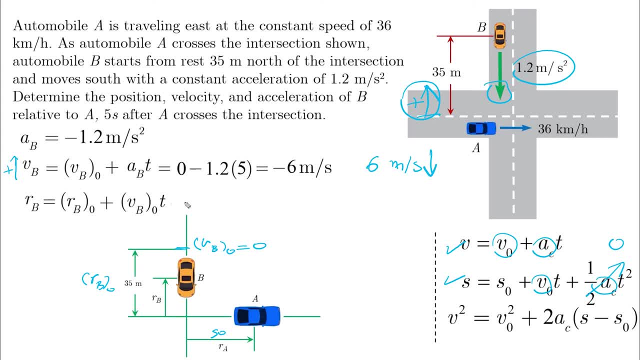 Is equal to RB naught plus VB naught T plus one-half AB T square. Again, this is positive up. So, assuming the origin is at the intersection, RB naught will be 35 meters in the positive direction. VB naught will be, as we said, equal to zero. 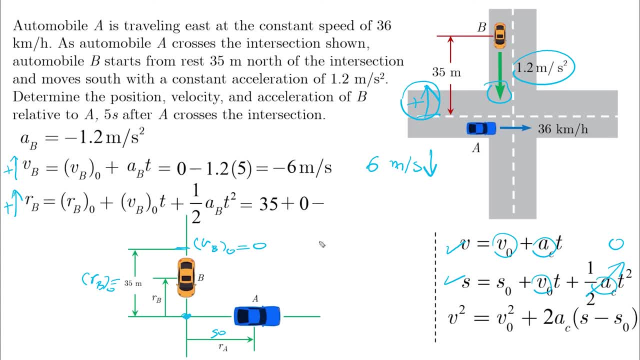 And this is plus one-half times minus 1.2.. And this is positive up Minus 1.2. as for the acceleration- or we can put this outside, as done here- times T square or 5 square, And this gives us 20 meters. 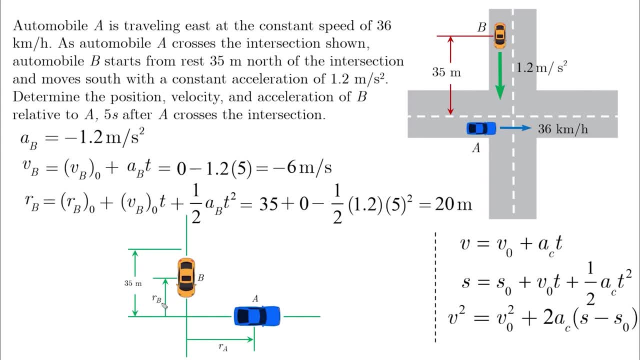 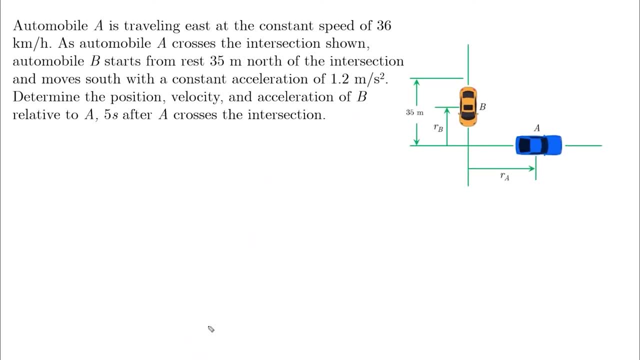 And this means that car B is now 20 meters from the origin, which is the intersection. And now that we have all the variables, after five seconds we can start with our B relative to A, Which is going to be RB, which is 20 meters in the positive J, minus RA, which is 50 meters. 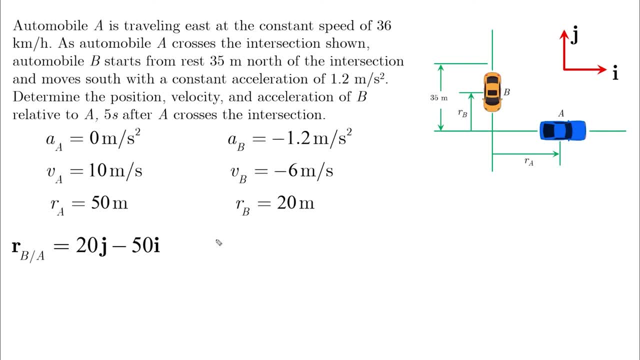 in the I direction And this leads to our magnitude and direction. And note that the direction is tan, inverse Y over X. As per this triangle, negative I with a positive J, And this becomes our angle. And for VB relative to A, we have the velocity of B in the negative J direction, minus the 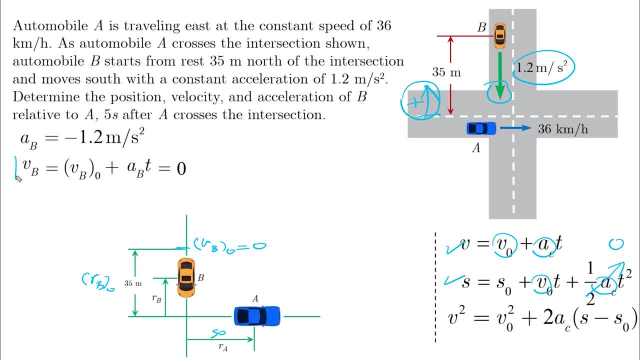 So we get zero from rest, Minus 1.2 multiplied by 5, which is the time, And this gives us minus 6 meters per second, or 6 meters per second in the downward direction. And as for the position RB, 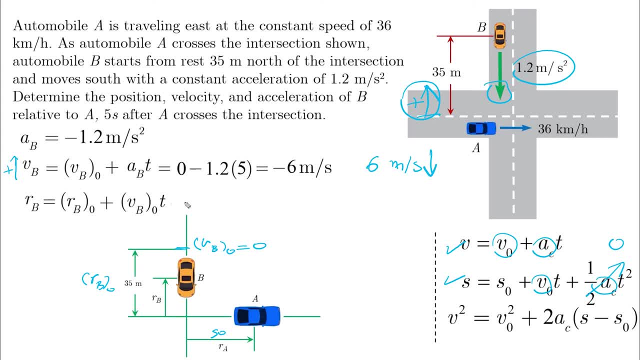 Is equal to RB naught plus VB naught T plus one half AB T square. Again, this is positive up. So assuming the origin is at the intersection, RB naught will be 35 meters in the positive direction. VB naught will be, as we said, equal to zero. 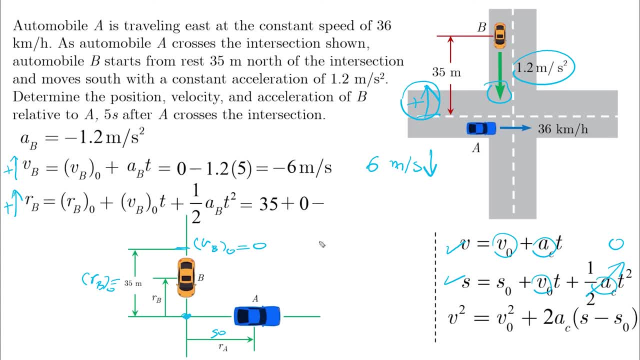 And this is plus one half times minus 1.2.. And this is positive up Minus 1.2,. as for the acceleration, or we can put this outside, as done here- times T square or 5 square And this gives us 20 meters. 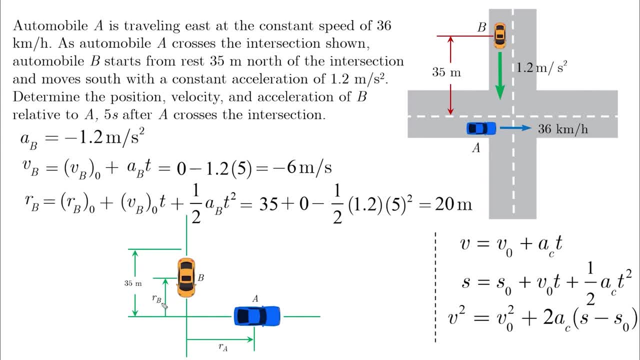 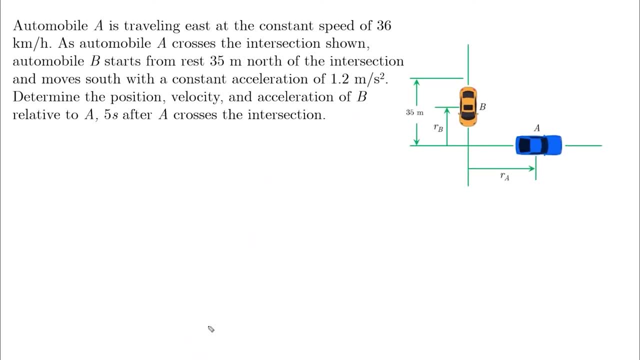 And this means that car B is now 20 meters from the origin, which is the intersection. And now that we have all the variables, after five seconds we can start with our B relative to A, Which is going to be RB, which is 20 meters in the positive J, minus RA, which is 50 meters. 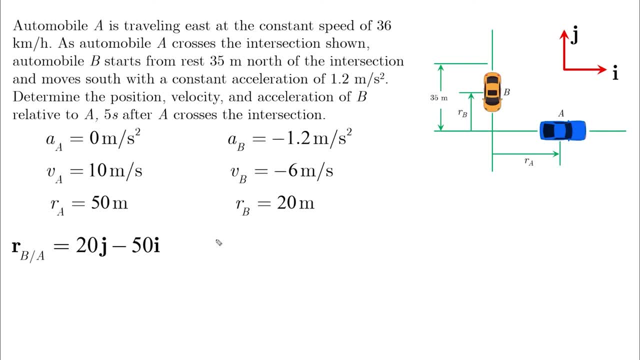 in the I direction And this leads to our magnitude and direction And note that the direction is tan, inverse Y over X. as per this triangle, negative I with a positive J, And this becomes our angle. And for VB relative to A, we have the velocity of B in the negative J direction, minus the 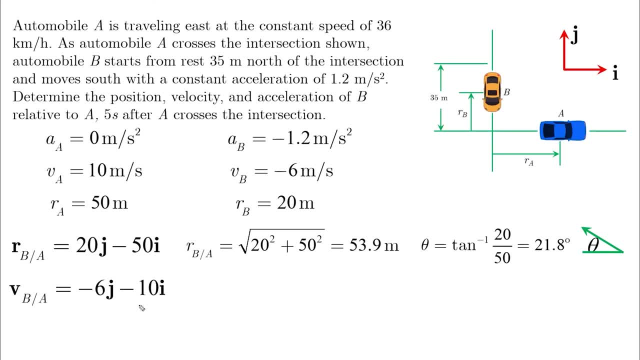 velocity of A, which is in the positive I direction, And if we take the magnitude and the direction becomes negative I with negative J, which leads to this angle. And finally, for the acceleration of B relative to A, we have negative I with negative J. 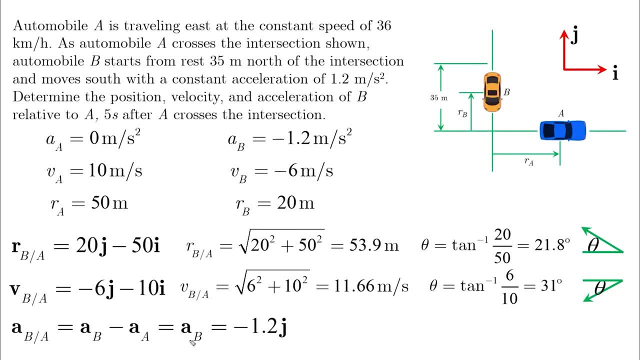 which leads to this angle. And if we take the magnitude and the direction, becomes negative, I with negative J, which leads to this angle. And finally, for the acceleration of B relative to A. since we don't have an acceleration of A, it's equal to zero. then AB relative to A will be equals to AB, which is minus.